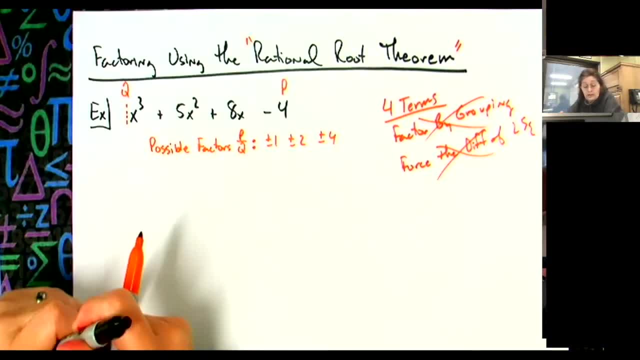 Okay, Now I'm trying to find something that goes into this: Okay, I don't want to do long division of polynomials, because that's absolutely horrible. Okay, So what I'm going to do is I'm going to use synthetic division. I know you did synthetic division in algebra two. All right, Synthetic. 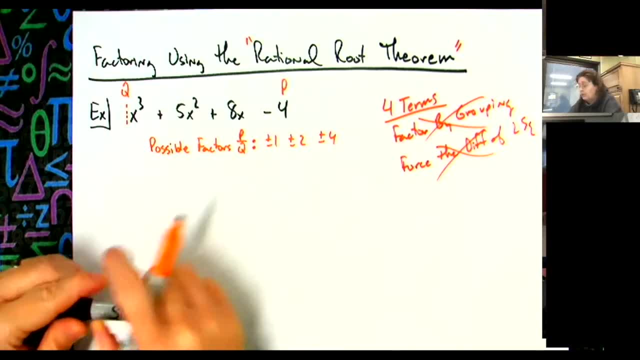 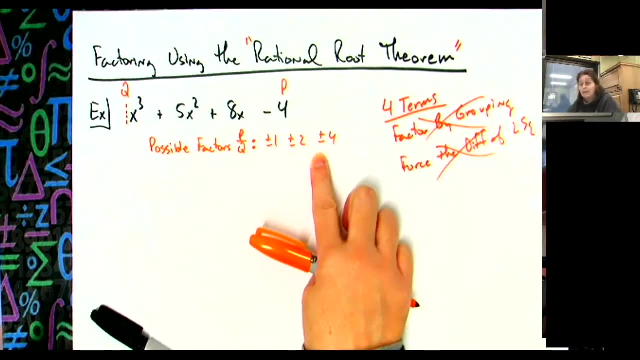 division because it goes really, really quick, All right, And then I'm going to. I've got a total of what? Two, four, six, I've got six choices. So if you are a bad guesser you might have to do synthetic division six times. Okay, But I'm 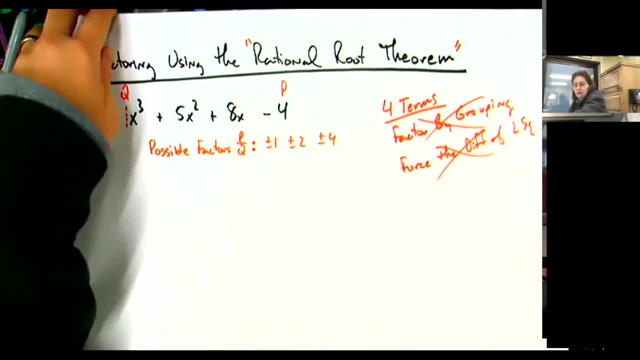 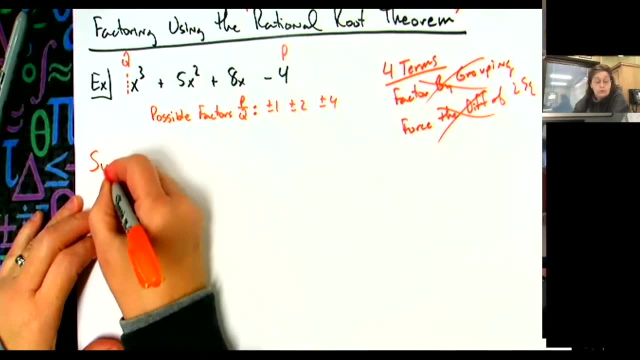 hoping you're not a bad guesser- And maybe, after two times, that you can get this to work, All right. And then I'm going to show you what it feels like to be frustrated and have to do it more than once. Okay, So let's go synthetic division, because that's what I'm going to do. 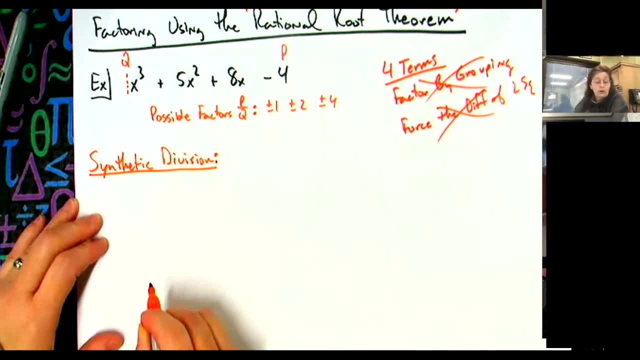 to make this shorter here. Okay, So let's try a four, All right. So I'm going to randomly pick one of those numbers. I'm going to try a four. All right, Now I'm picking four from here. I'm going to take all my coefficients and write them. 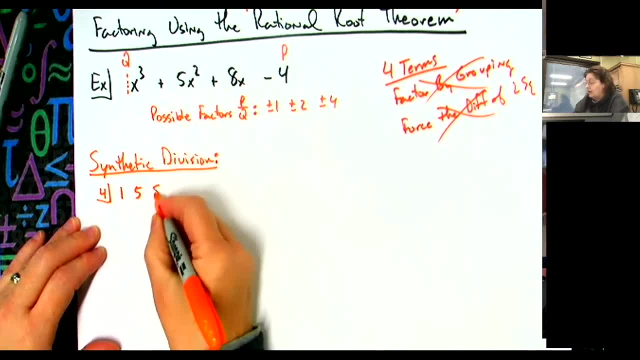 down. So I got a one, then I got a five, then I got an eight, then I got a negative four. Synthetic division, hopefully, is going to start to come back to you. This one comes straight down: One times four is four. Don't let me screw up the arithmetic. Four plus five is going to be nine. 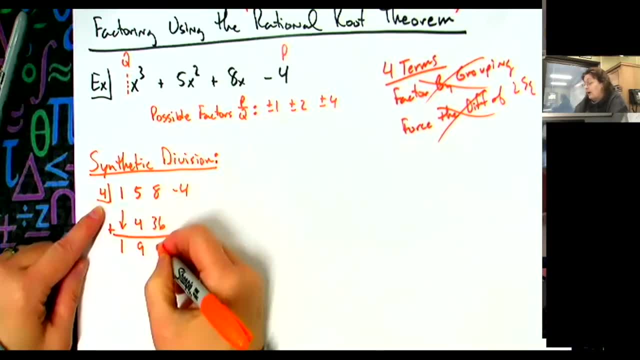 Nine and four is 36.. When I add going down, what's that going to be like 44. Holy crap. And then 44 times 44. I have no freaking clue what that is off the top of my head And it's too early in the morning for me to try to do it. I get like a 176 and then 176. And that. 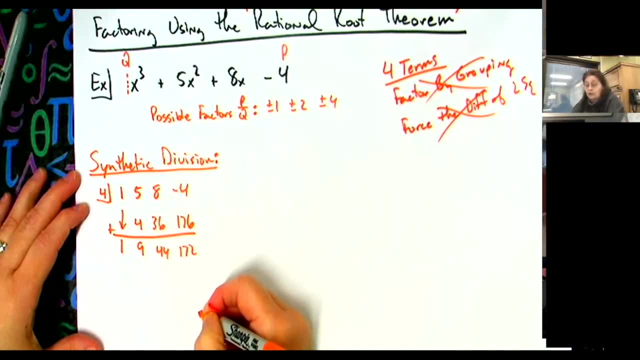 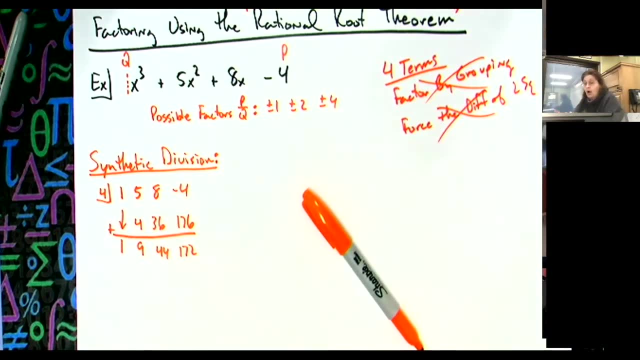 negative four is going to give me a 172.. All right, Guess what It didn't work. Okay, I did not get a zero here. Okay For it, my synthetic division. I know when I pick the right number, when I get a. 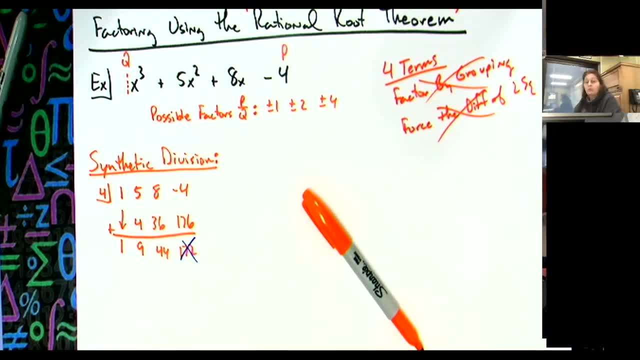 zero right here. well, that's not zero. So, picking four: what's the wrong guess? Okay, That's okay. I'm not going to get frustrated, All right, I'm just going to come up here and I'm going to try it. 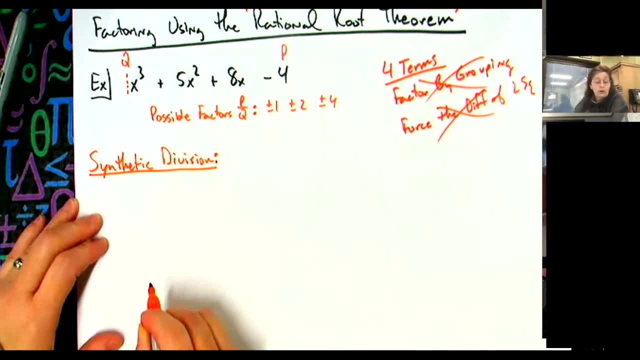 to make this shorter here. Okay, So let's try a four, All right. So I'm going to randomly pick one of those numbers. I'm going to try a four. All right, Now I'm picking four from here. I'm going to take all my coefficients and write them. 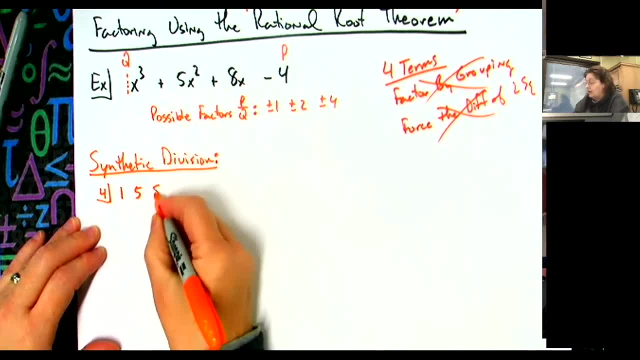 down. So I got a one, then I got a five, then I got an eight, then I got a negative four. Synthetic division, hopefully, is going to start to come back to you. This one comes straight down: One times four is four. Don't let me screw up the arithmetic. Four plus five is going to be nine. 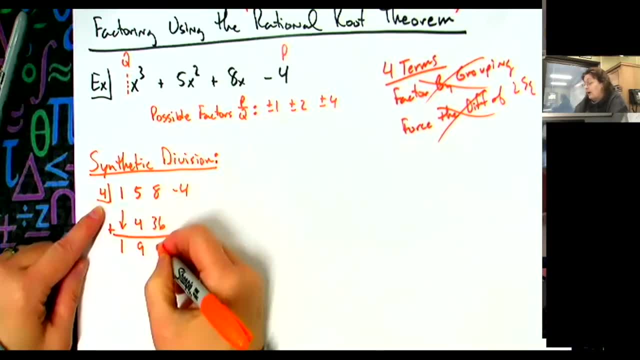 Nine and four is 36.. When I add going down, what's that going to be like 44. Holy crap. And then 44 times 44. I have no freaking clue what that is off the top of my head And it's too early in the morning for me to try to do it. I get like a 176 and then 176. And that. 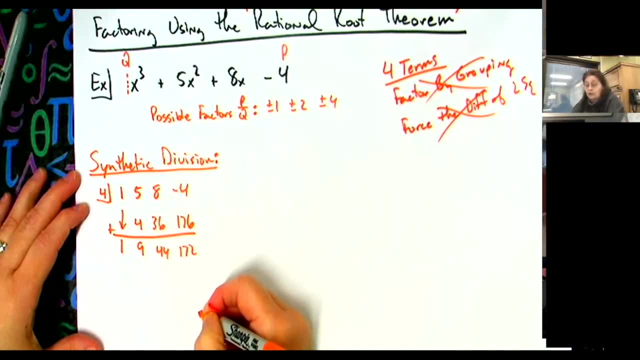 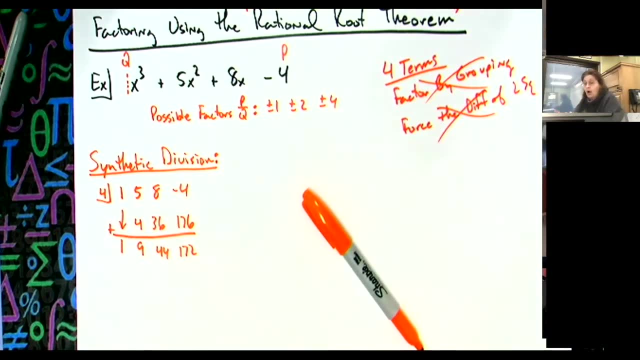 negative four is going to give me a 172.. All right, Guess what It didn't work. Okay, I did not get a zero here. Okay For it, my synthetic division. I know when I pick the right number, when I get a. 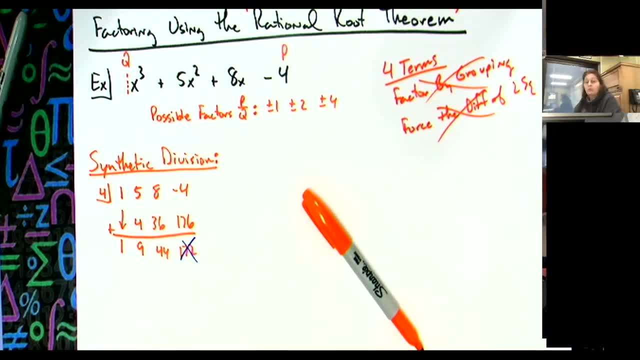 zero right here. well, that's not zero. So, picking four: what's the wrong guess? Okay, That's okay. I'm not going to get frustrated, All right, I'm just going to come up here and I'm going to try it. 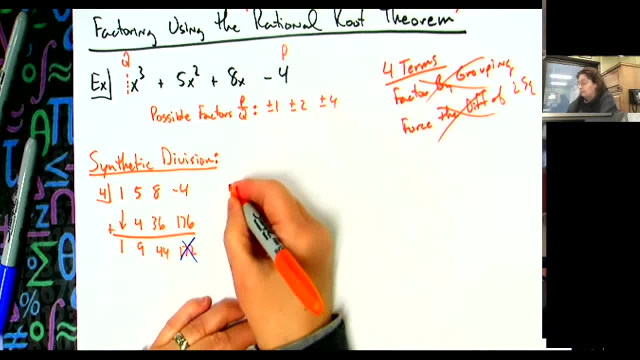 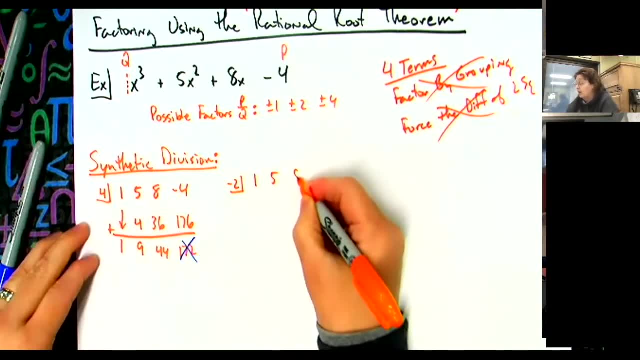 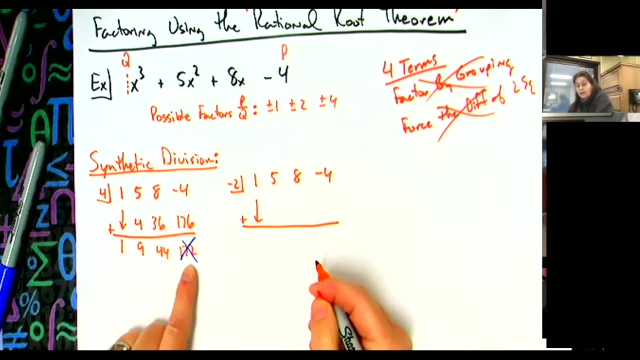 again. Okay, So this time let's pick a negative two. All right, So I pick negative two for my list. Then I'm going to do a one and my five and my eight and my negative four. Those are my coefficients for my original problem And I'm going to try again. All right, I'm trying to get. 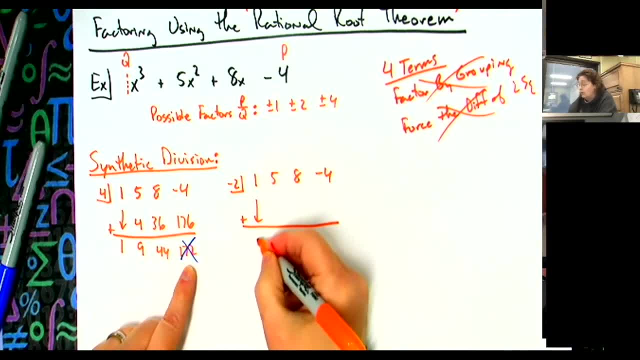 a remainder of zeros What I'm trying to do on this. So I'm going to drop my one. one times negative. two, three. two times the negative Negative. two times three is six. That's going to be. what am I doing wrong? I'm doing something. 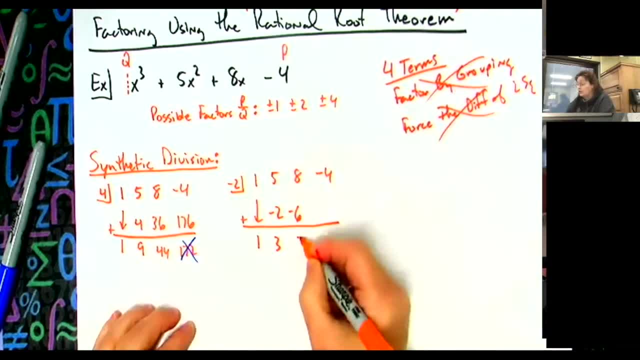 wrong here. That'd be a negative six. There we go, And then I'm going to get a two and then two times negative two is going to be. I did something wrong again. What am I doing wrong? I'm doing something wrong, So I'm going to check my math. Negative two, three negative six: two negative. 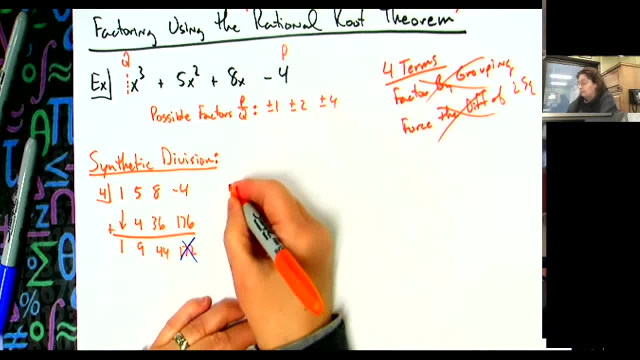 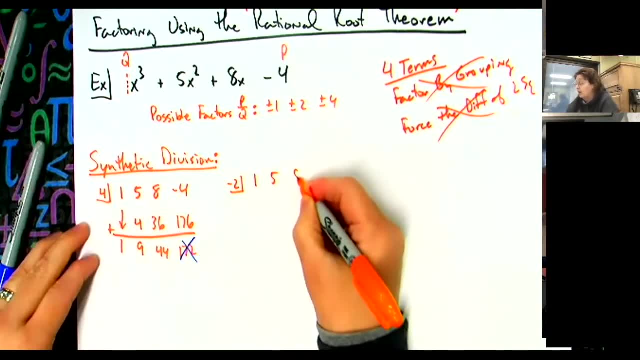 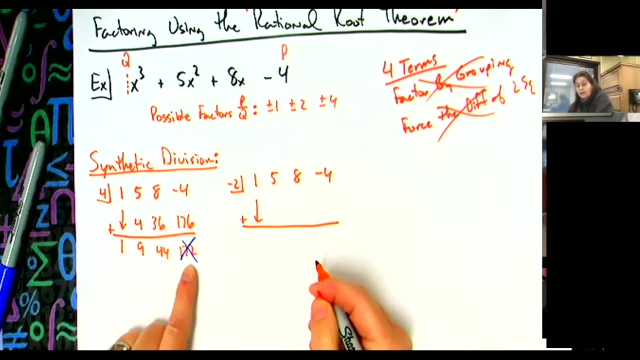 again. Okay, So this time let's pick a negative two. All right, So I pick negative two for my list. Then I'm going to do a one and my five and my eight and my negative four. Those are my coefficients for my original problem And I'm going to try again. All right, I'm trying to get. 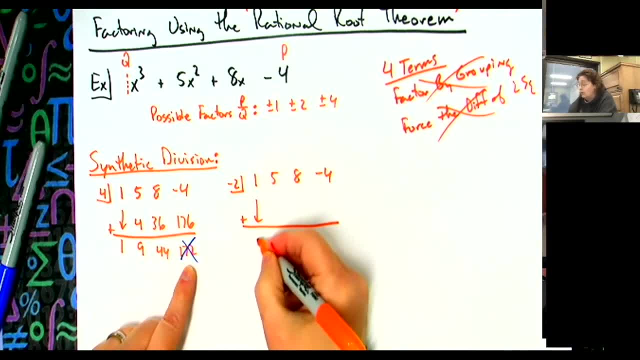 a remainder of zeros What I'm trying to do on this. So I'm going to drop my one. one times negative. two, three. two times the negative Negative. two times three is six. That's going to be. what am I doing wrong? I'm doing something. 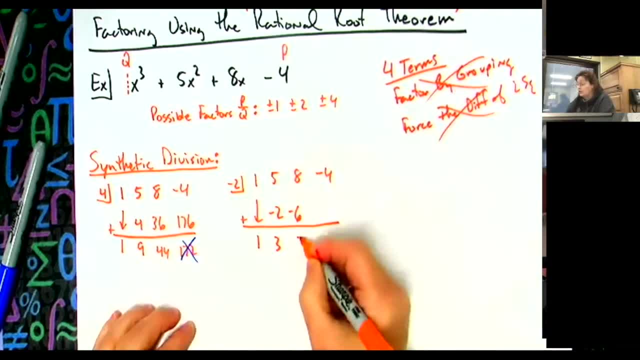 wrong here. That'd be a negative six. There we go, And then I'm going to get a two and then two times negative two is going to be. I did something wrong again. What am I doing wrong? I'm doing something wrong, So I'm going to check my math. Negative two, three negative six: two negative. 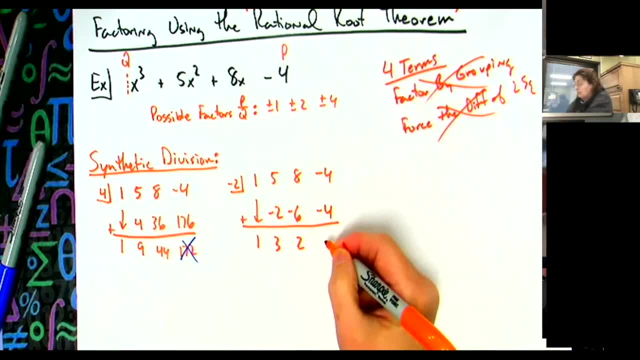 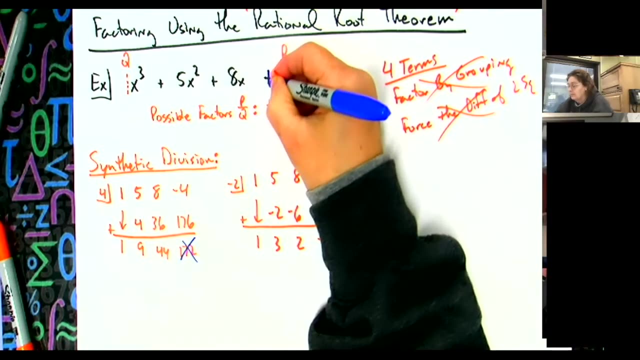 four: Okay, That's negative eight, All right. The reason this isn't working is because I copied my problem down wrong to begin with. All right, I knew I wasn't doing something wrong. Okay, Let's go back and fix. All right, This really needs to be a plus sign right here. All right. So if this is a 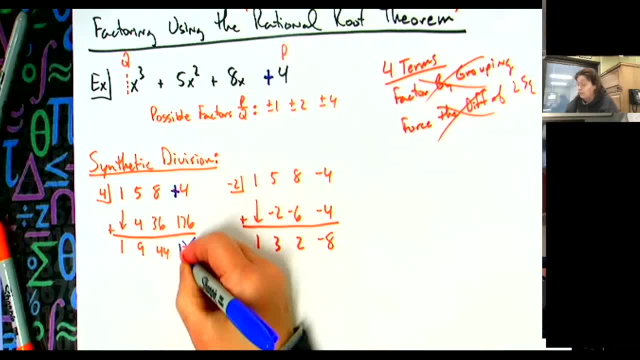 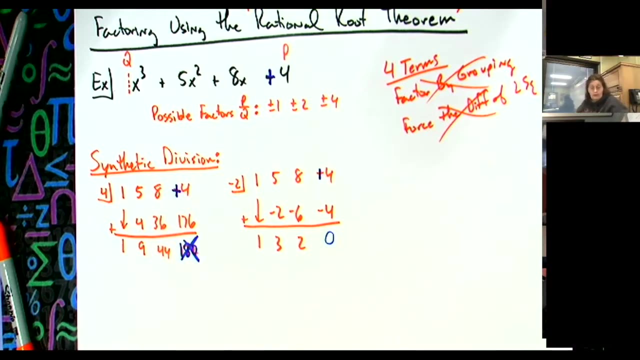 plus. all right, then that's like 180,, but it still didn't work, So throw it out. All right, That would make this a plus, That would make this a zero. Helps when I copy the problem down right. guys, I apologize for that. Okay, So when I copied the problem down right and that became a positive. 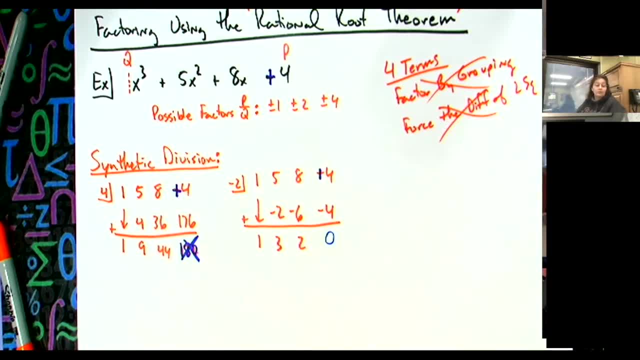 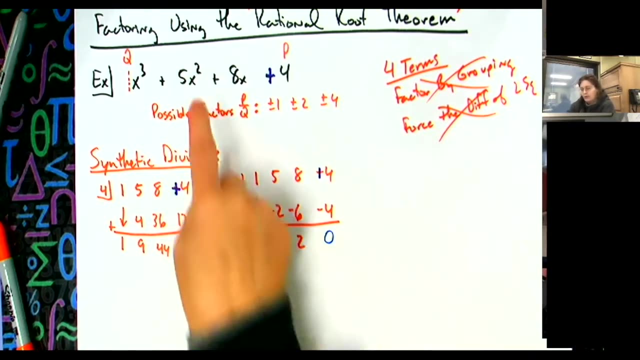 four, all right. I still have factors of plus or minus one, plus or minus two, plus or minus four, All right. Now I got a zero here, All right. What that tells me is that X plus two is a binomial factor. that goes into this. All right, Because negative two is a root. 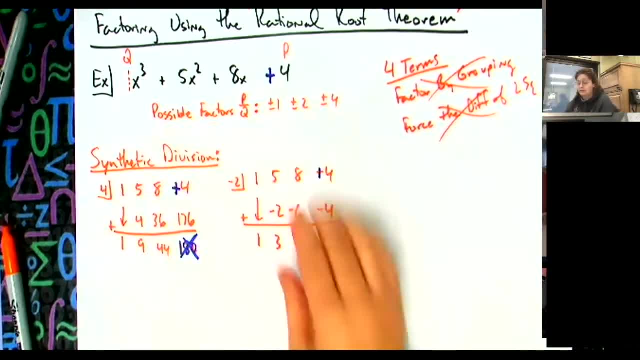 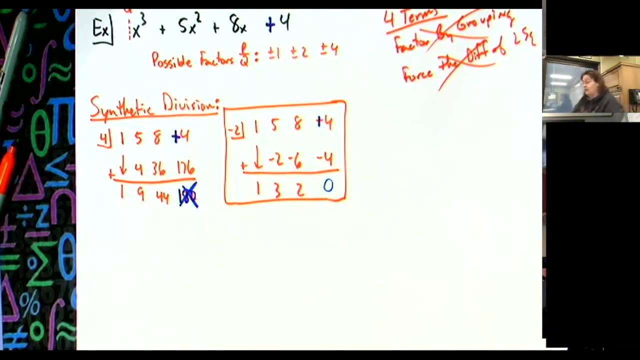 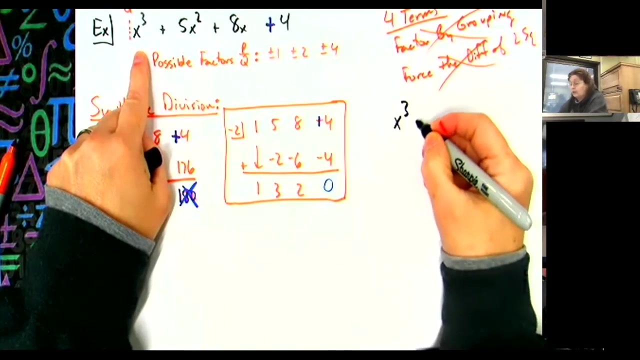 Okay, So when I do this synthetic division, I am looking for one, one of these that gives me a zero remainder. Okay, Now, from there I can conclude some things. All right, I'm going to start over here and rewrite this. Okay, So, X to the third plus five. 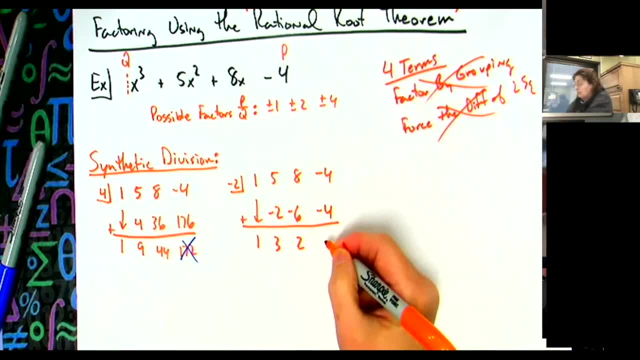 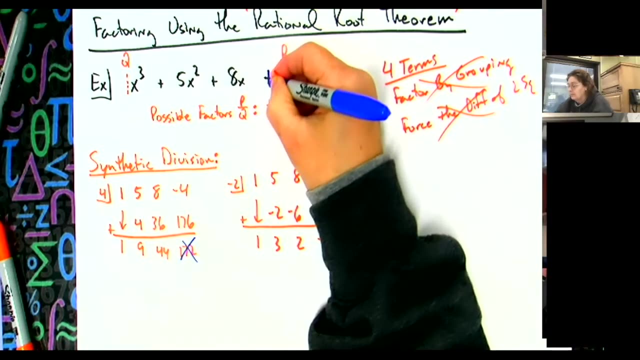 four: Okay, That's negative eight, All right. The reason this isn't working is because I copied my problem down wrong to begin with. All right, I knew I wasn't doing something wrong. Okay, Let's go back and fix. All right, This really needs to be a plus sign right here. All right. So if this is a 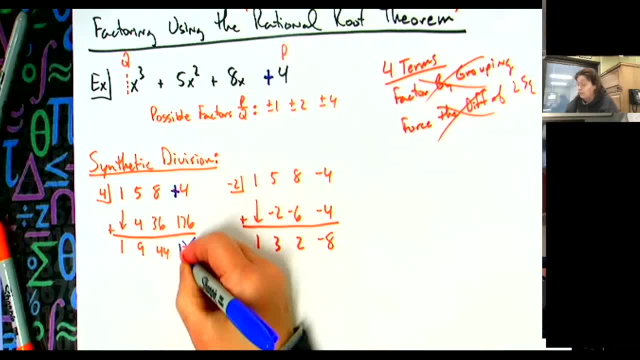 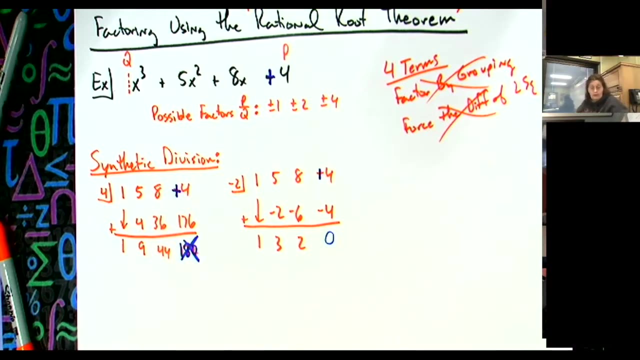 plus. all right, then that's like 180,, but it still didn't work, So throw it out. All right, That would make this a plus, That would make this a zero. Helps when I copy the problem down right. guys, I apologize for that. Okay, So when I copied the problem down right and that became a positive. 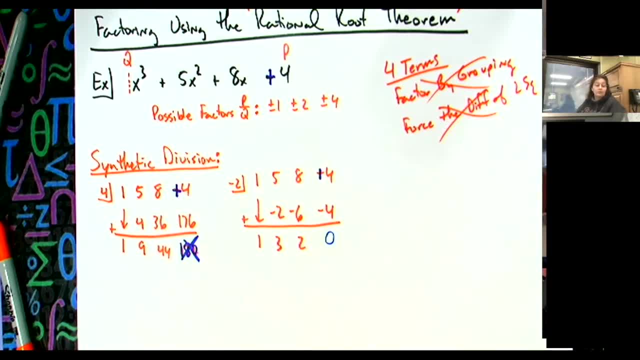 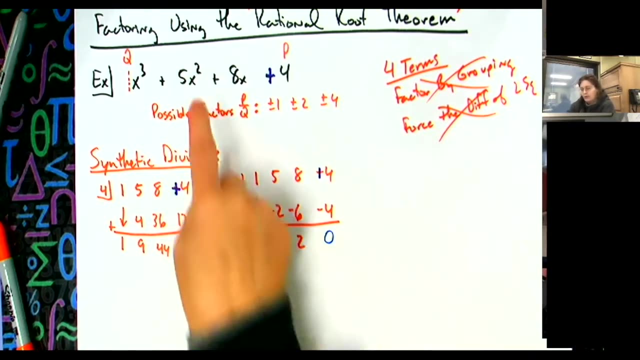 four, all right. I still have factors of plus or minus one, plus or minus two, plus or minus four, All right. Now I got a zero here, All right. What that tells me is that X plus two is a binomial factor. that goes into this. All right, Because negative two is a root. 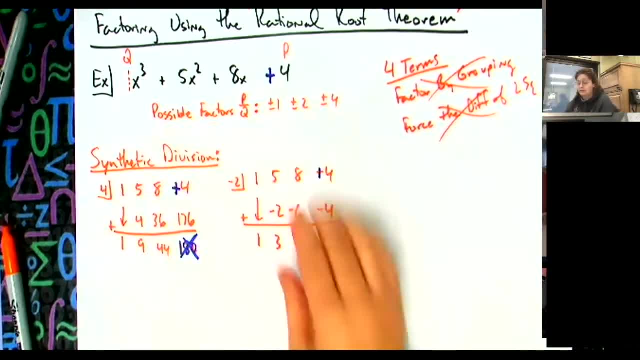 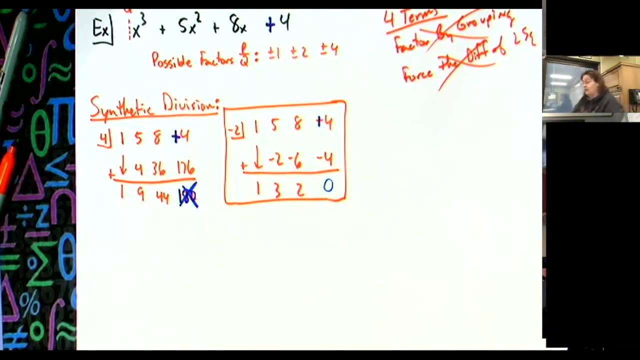 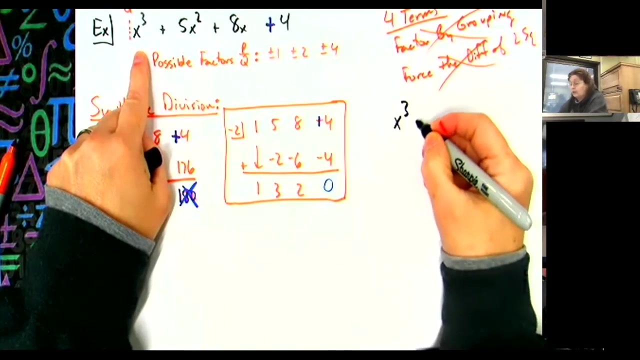 Okay, So when I do this synthetic division, I am looking for one, one of these that gives me a zero remainder. Okay, Now, from there I can conclude some things. All right, I'm going to start over here and rewrite this. Okay, So, X to the third plus five. 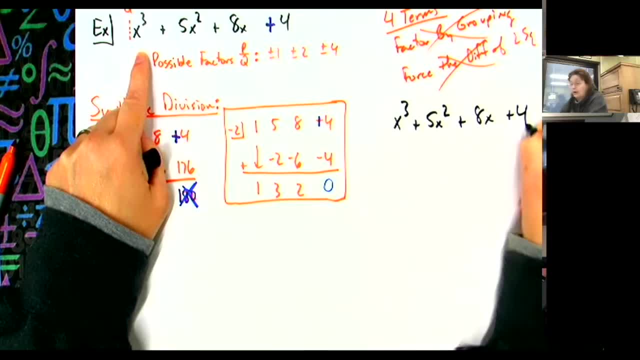 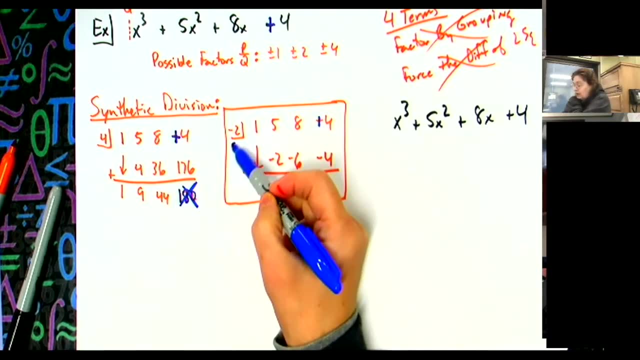 X squared plus eight, X plus my four. Okay, That's my original polynomial. right Now I'm going to come over here and look at my synthetic division. All right, This right here tells me this is a minus two. So that tells me I have an X plus two as a factor. Okay, Because 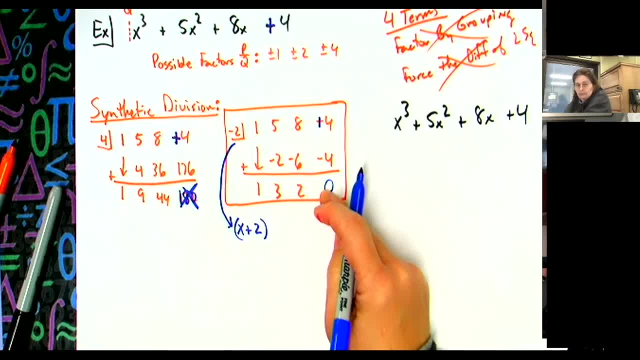 I did it, I divided it in, I did my long division, but I did shortcut. with synthetic division. I got a remainder of zero. So it is a factor All right. And then from here I can come up with, if you remember how synthetic division works. you start here. this is your plane number And 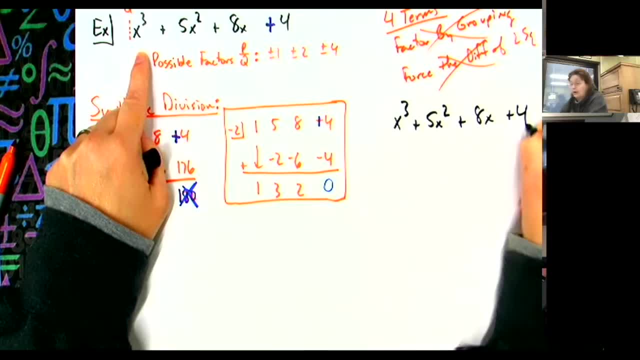 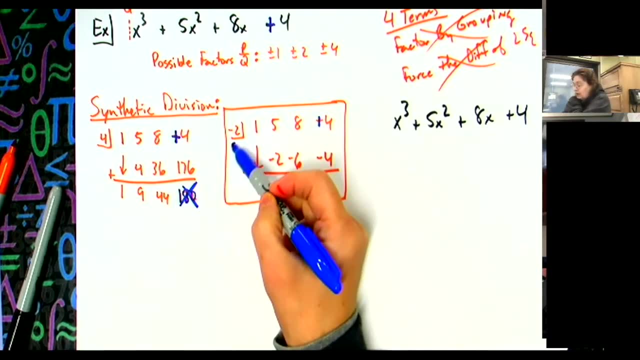 X squared plus eight, X plus my four. Okay, That's my original polynomial. right Now I'm going to come over here and look at my synthetic division. All right, This right here tells me this is a minus two. So that tells me I have an X plus two as a factor. Okay, Because 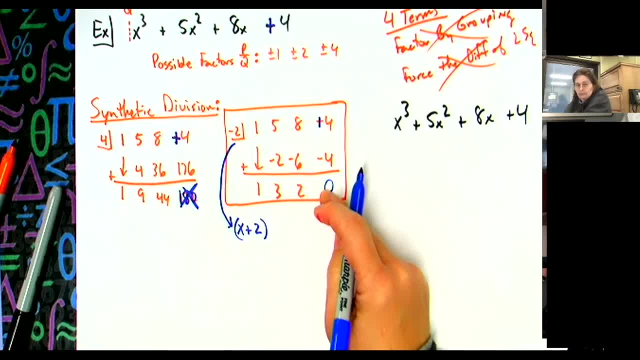 I did it, I divided it in, I did my long division, but I did shortcut. with synthetic division. I got a remainder of zero. So it is a factor All right. And then from here I can come up with, if you remember how synthetic division works. you start here. this is your plane number And 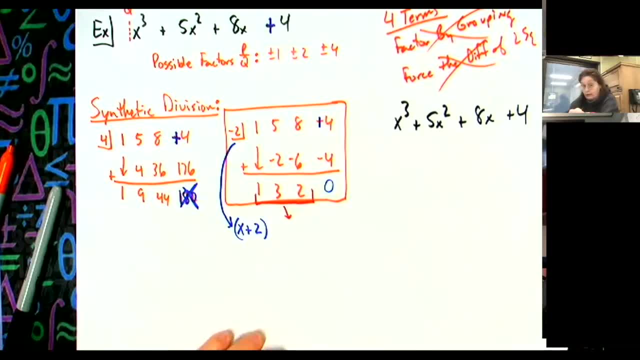 then this is your X term, And then this is your X term, And then this is your X term, And then this is your X squared term. You go right to left. You actually go backwards here. So from there I get an X squared one coefficient plus a three, X plus a two. So this one, three and two gives. 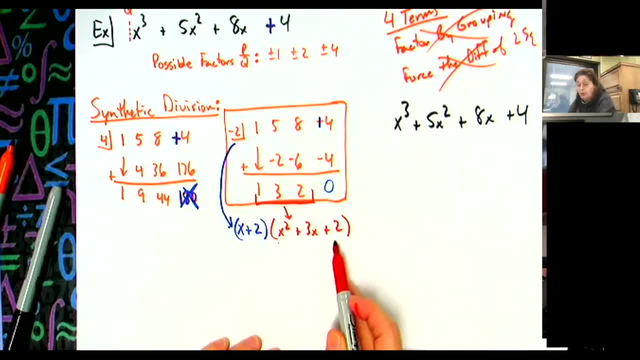 me my one, X squared plus three X plus two, It gives me a trinomial. All right, So I didn't have to do long division. I did this, And from that synthetic division I get this. All right. Now, what is this? This is: 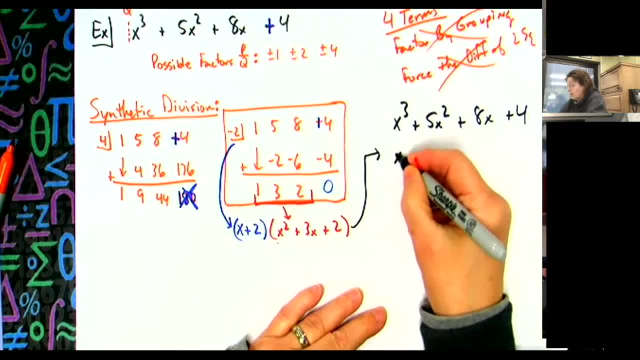 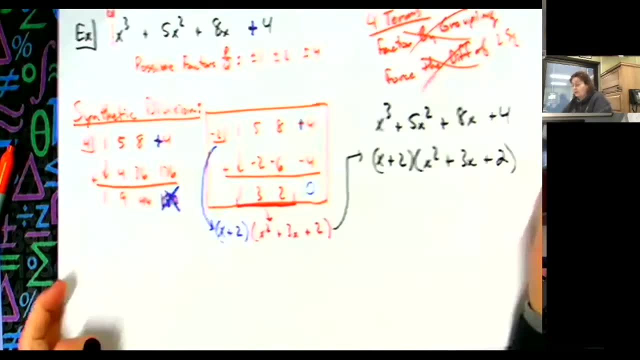 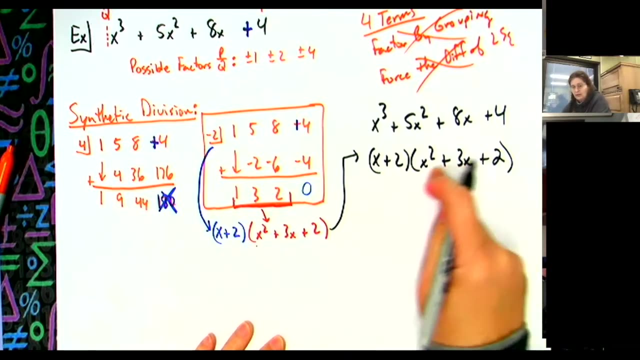 the A factored line for this. So X plus two, and then X squared plus three, X plus two. All right, So this four term polynomial factors to this, and I was able to get to this by doing synthetic division. Okay, Now, what is this? This is a trinomial, and I should maybe be able to factor. 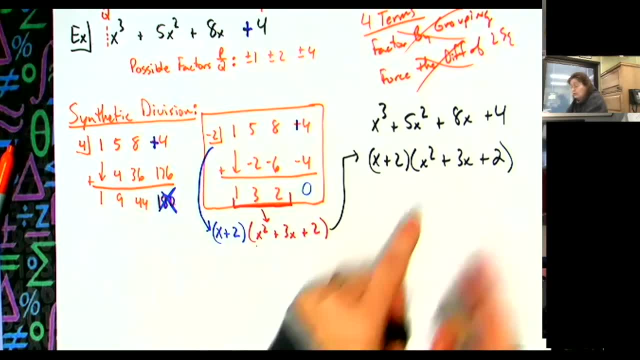 this. This is going to give me a two and a one, which is going to give me a two and a one, And this is going to give me a three in the middle. So now I'm just going to keep factoring like normal. So this X plus two is going to stay. I'm going to guess and check this one. 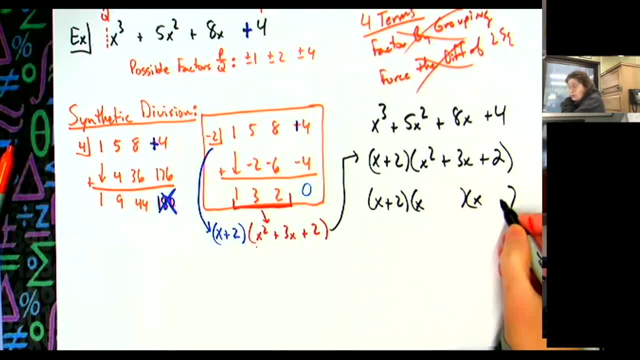 into an X and an X. I've got all plus signs. The only thing that multiplies together is two is two times one. I'm going to put a plus in there, and I'm going to put a plus in there. Okay, Now that. 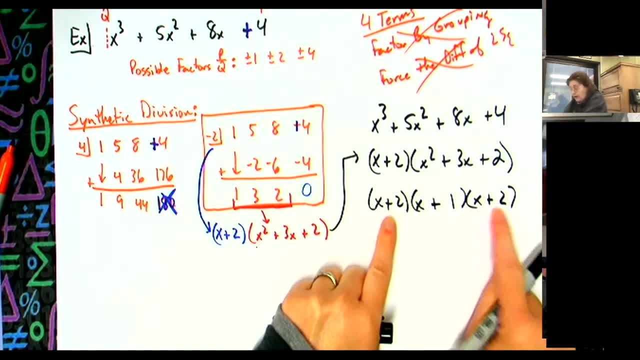 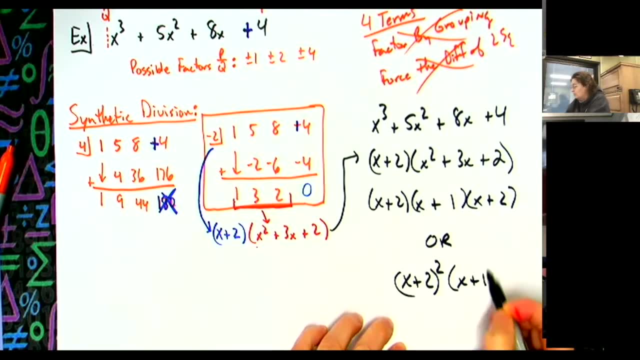 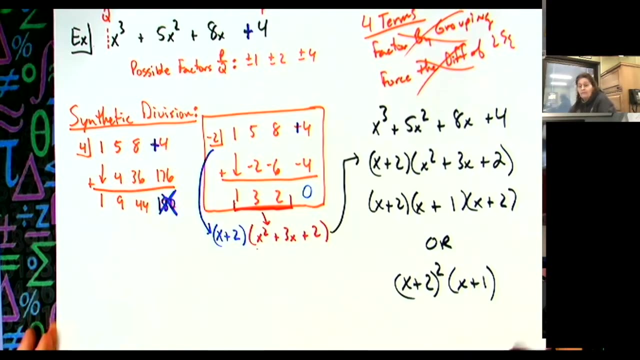 is completely factored there. but notice, these two terms do match. If I'm really fancy and really good, I could write it as an X plus two to the second power times, an X plus one. All right, So I have now been able to factor this polynomial that had four terms in it. 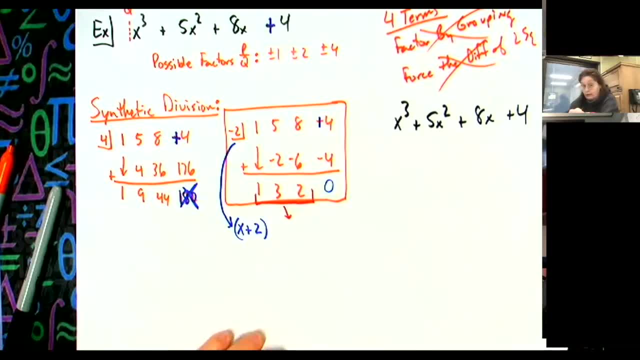 then this is your X term, And then this is your X term, And then this is your X term, And then this is your X squared term. You go right to left. You actually go backwards here. So from there I get an X squared one coefficient plus a three, X plus a two. So this one, three and two gives. 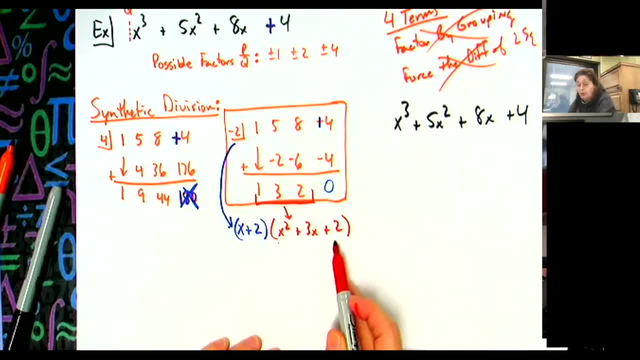 me my one, X squared plus three X plus two, It gives me a trinomial. All right, So I didn't have to do long division. I did this, And from that synthetic division I get this. All right. Now, what is this? This is: 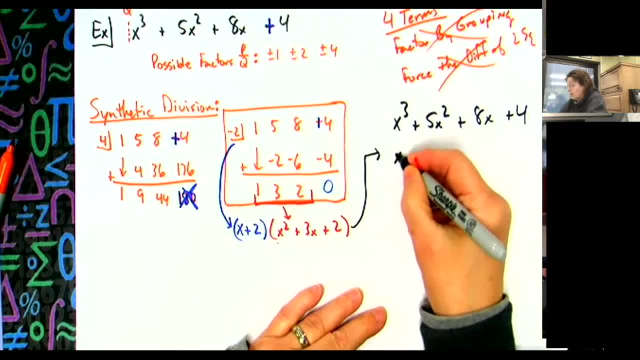 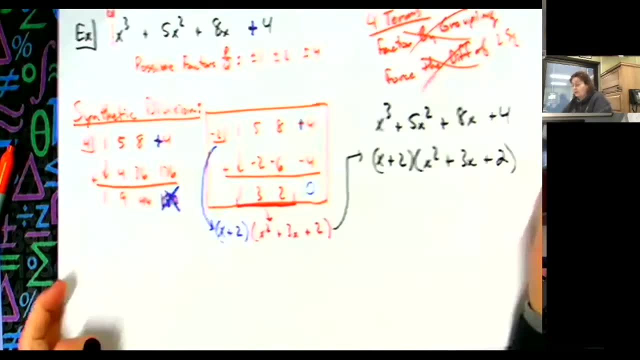 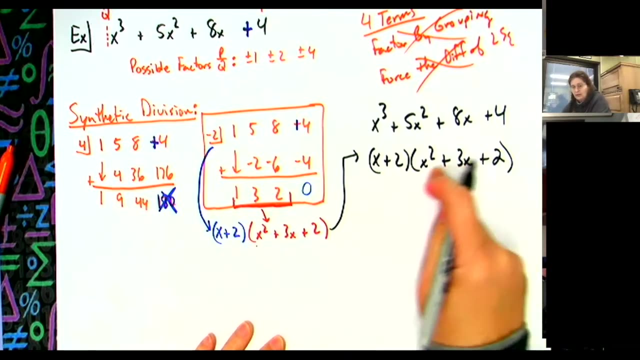 the A factored line for this. So X plus two, and then X squared plus three, X plus two. All right, So this four term polynomial factors to this, and I was able to get to this by doing synthetic division. Okay, Now, what is this? This is a trinomial, and I should maybe be able to factor. 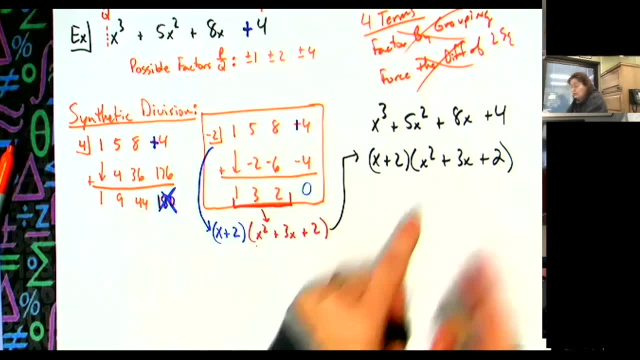 this: This is going to give me a two and a one, which is going to give me a two and a one. This is going to give me a three and a middle. So now I'm just going to keep factoring like normal. 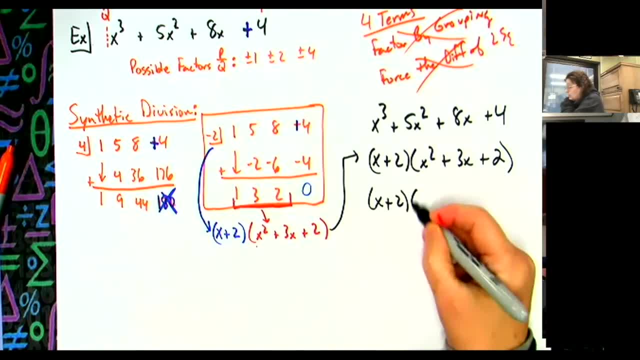 So this X plus two is going to stay. I'm going to guess and check this one into an X and an X. I've got all plus signs. The only thing that multiplies together is two is two times one. I'm going to put a plus in there and I'm going to put a plus in there. 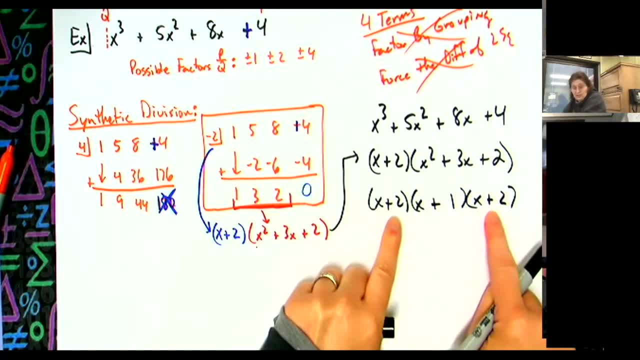 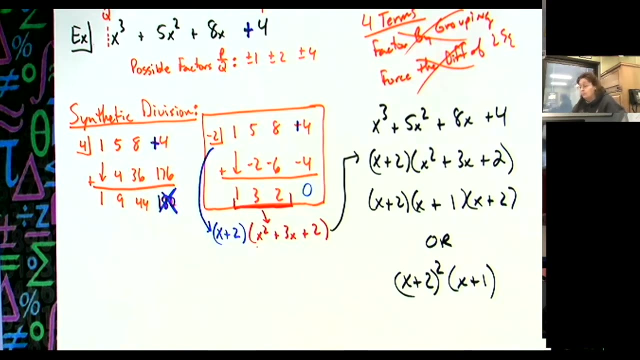 Okay, Now that is completely factored there. but notice, these two terms do match. If I'm really fancy and really good, I could write it as an X plus two to the second power times, an X plus one. All right, So I have now been able to factor this polynomial that had four terms in it. 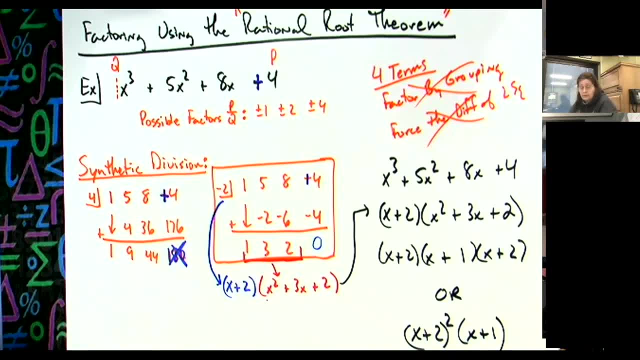 but I didn't do it by factor, by grouping, because that didn't work, and I didn't do it by forcing the difference of two squares, because that didn't work. So I had to rely on the rational root theorem to be able to get to there. 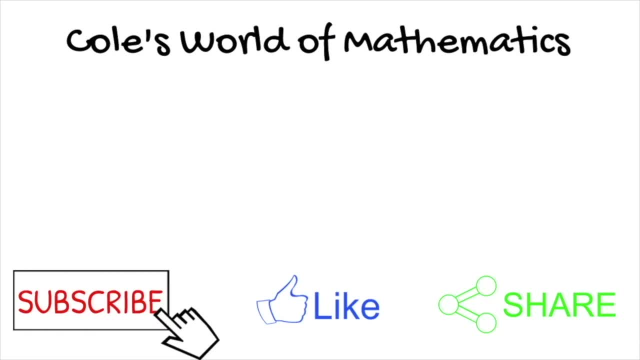 Here's where I'm going to add some more Good. See you in seven years.